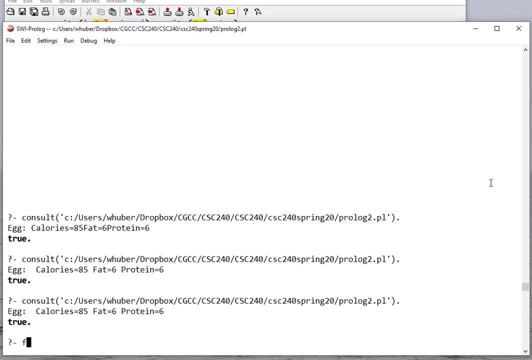 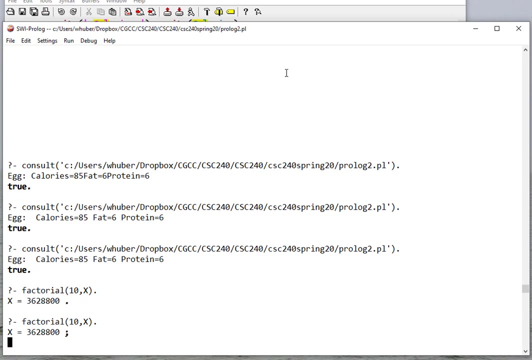 So let's see how that works. Now we can see. I get the answer. Now it does prompt me for an additional answer, And this is probably going to go on forever, So I need to stop that, And the reason for that is is that eventually, 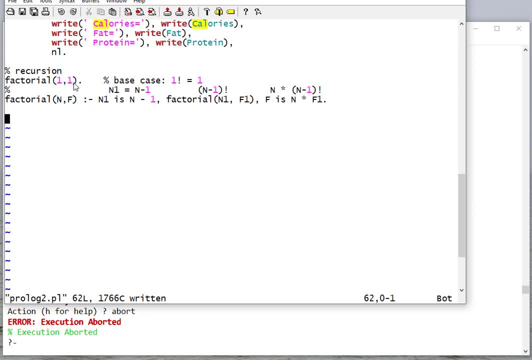 when I reject this base case, then it says: OK, well, I'll subtract 1 from n. So actually to be safe, it might be a good idea to say n is greater than 1.. And so that sort of ensures that I don't have this infinite loop. 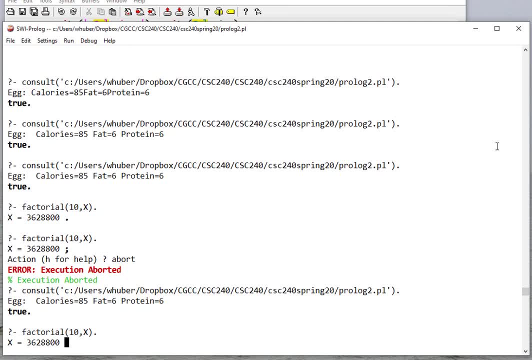 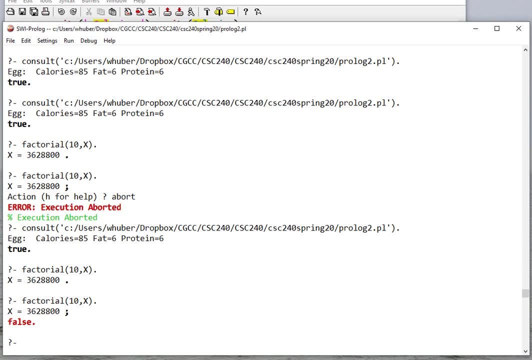 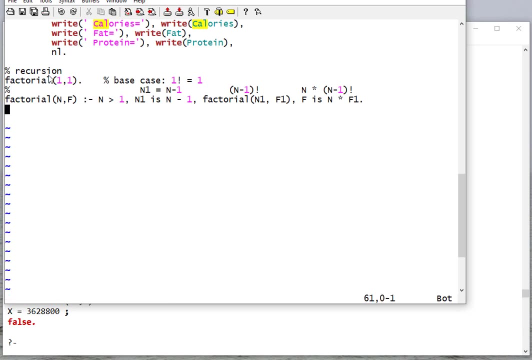 So now let's consult again. And now, if I ask it for additional answers, it says false, It can't find anything else. So the way recursion works is: remember that prolog search is from top down, So it's going to see this rule. 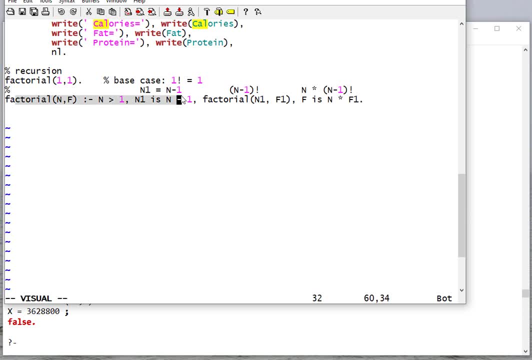 If that doesn't work, then it'll try to find another rule, And so it'll do this recursive case Here. I make a recursive call, And it will try to unify n1 and f1 before it proceeds on to the next computation. 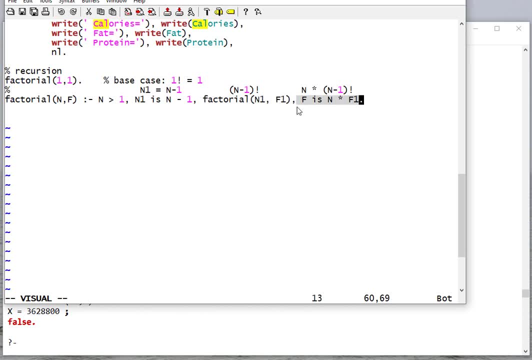 But once it does, then it'll come here And check to see or try to calculate f based on n and f1.. OK, so now let's look at a recursive definition, not just of addition and multiplication, like we did with scheme. 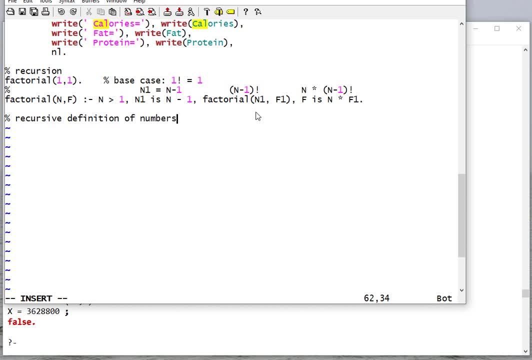 But let's actually do a recursive definition of numbers themselves. 0 is a number, Then the successor of a number is a number, And notice, here we're treating the successor as a function. Any number can be represented this way because, for example, 2 is the successor of 1,. 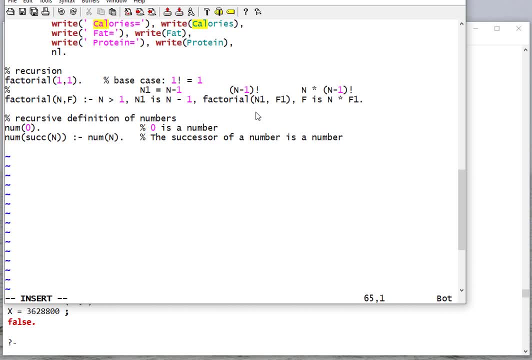 which is the successor of 0. So it's a number. So to add two numbers first off my base case: if I add 0 to x, I just get x, And that's also true if, if I add 0 to a number. 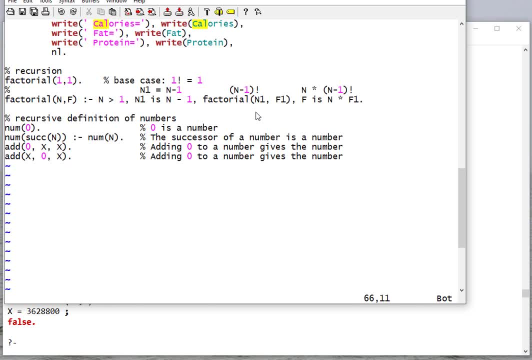 I still get x, But I need both rules because I don't know where the 0 is going to be. If I add the successor of x and y, I'm going to get the successor of z, where I'm adding x and y to get z. 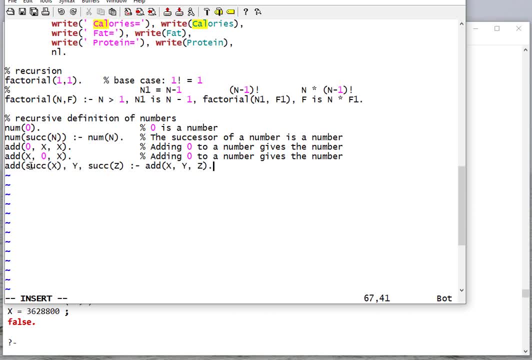 So the way this works is, if I add some successor of x to y, then that means the result is the successor of adding x to y And, just like before, I also could have this second number be a number with a successor. So let's consult. 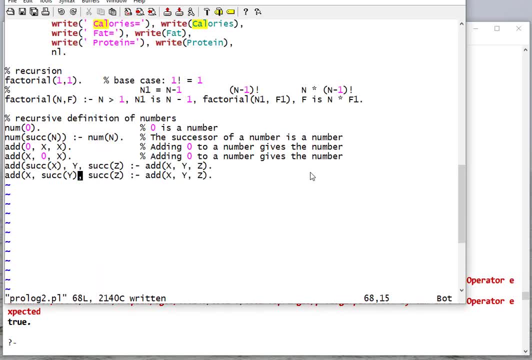 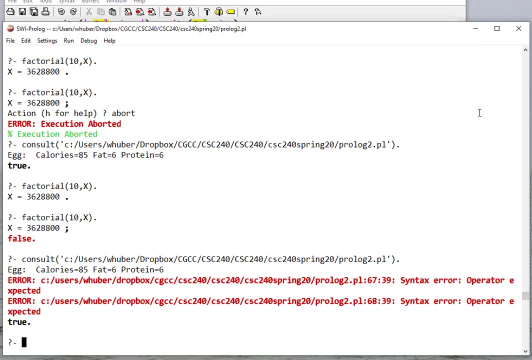 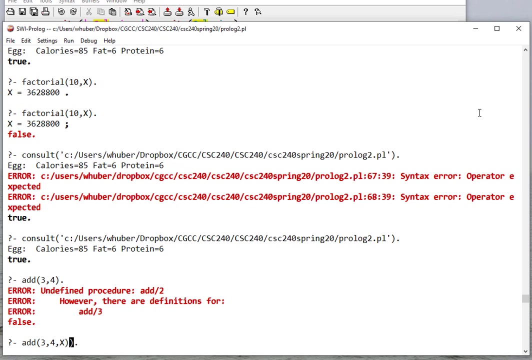 And we have a syntax error on line 68, column 39.. Ah, I don't have a closing parentheses here. That should fix it. Now I can't add 3 and 4 and to get x, But I can add. 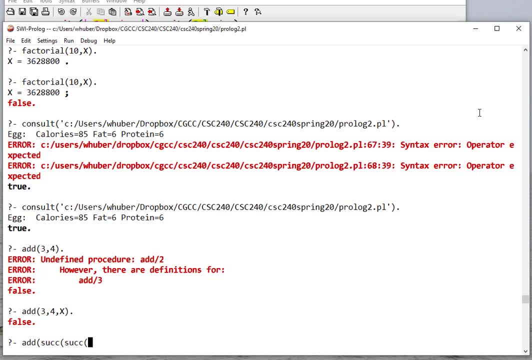 the successor of the successor of the successor of 0.. And I need 1,, 2,, 3 closing parameters. That's 3.. And this is 4.. 1,, 2,, 3,, 4.. And 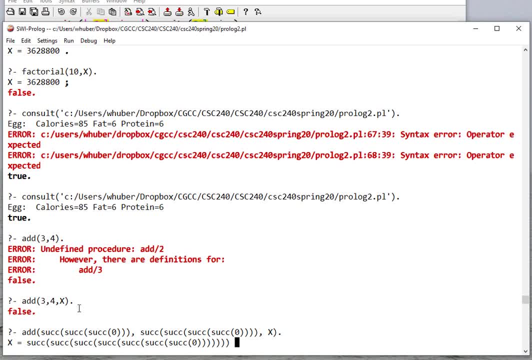 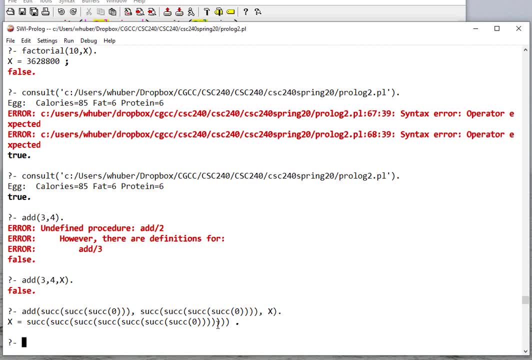 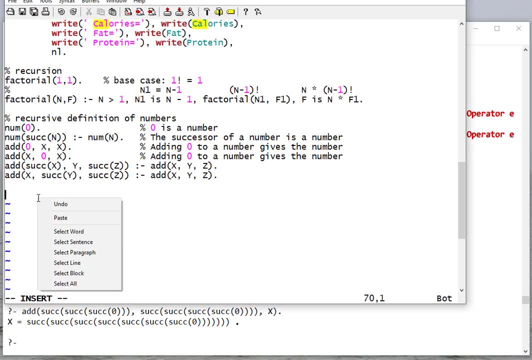 I'm doing addition using just recursion. There's nothing else. There's not even any arithmetic operations involved here. Literally recursion is the only thing I'm doing. Let's write a few more recursive rules, And here we're going to set up a family. 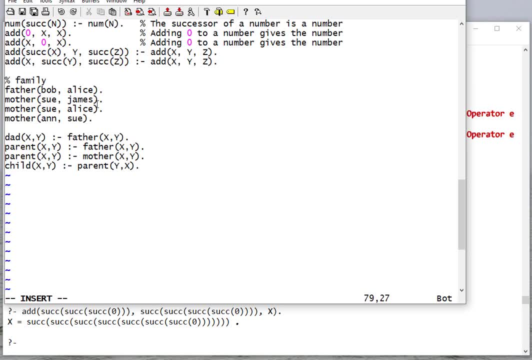 set of facts. So Bob is the father of Alice, Sue is the mother of James, Sue is the mother of Alice And Ann is the mother of Sue. Then we have some rules: Dad x- y. if father x y. 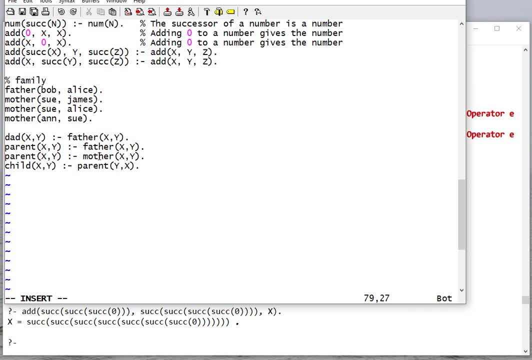 Parent x y if father x y, Or parent x y if mother is of x y. So that means that whether x is the mother or father of y parent x y if father x y, They're the parent. 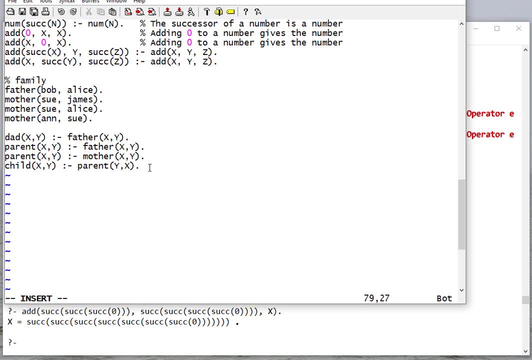 Either one rules And then the child reverses the parent relationship. Now let's say we want to do an ancestor rule, So A is the ancestor of D if A is the parent of D. Now that just gives us one level. 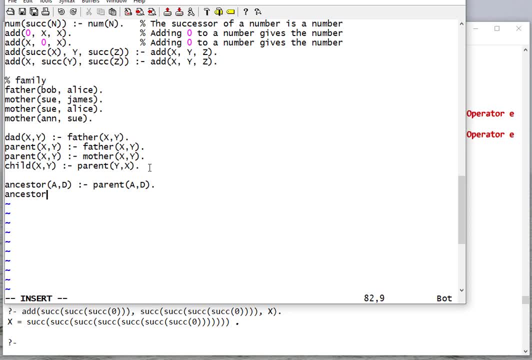 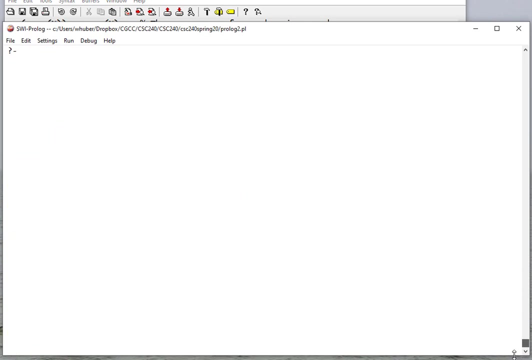 So to get the additional levels of being an ancestor, we'll have a recursive rule: A is the ancestor of D, If ancestor of A x, that x is the ancestor of A. So let's try that rule and see what happens. 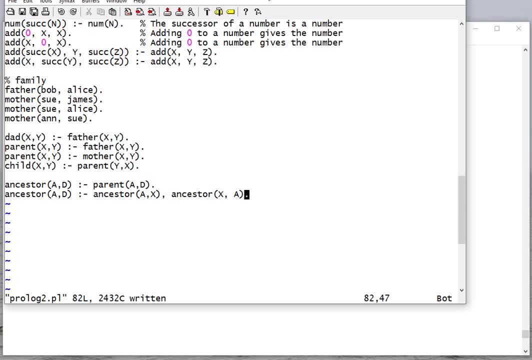 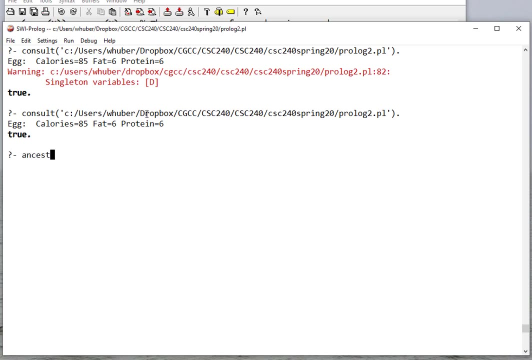 And I have a singleton variable, So let's fix that, because I definitely don't want that. Ah, this should be D. x is the ancestor of D. Okay, so we've consulted. Now let's ask if Alice or Bob is the ancestor of Alice. 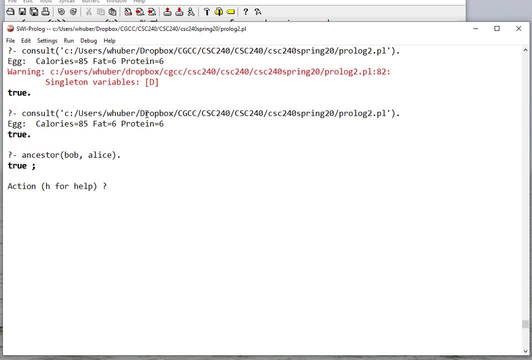 That's true, But then notice when I rejected, that it kind of hung for a while. So let's try this. How about ancestor James now, if you go back and look at the code and is the mother of sue and sue is? 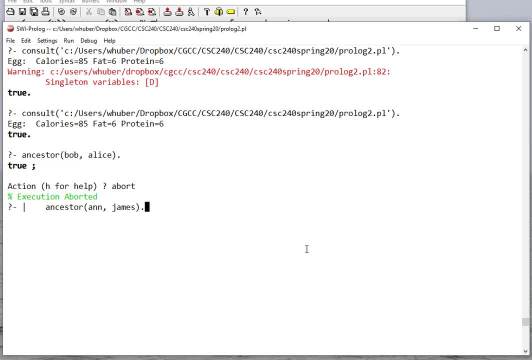 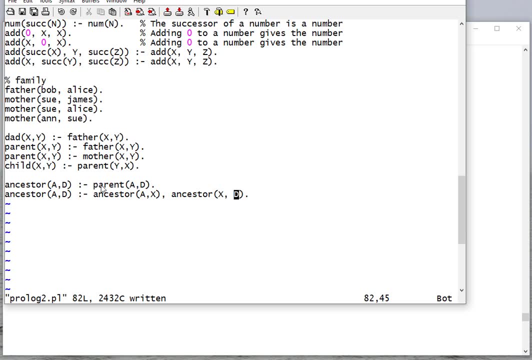 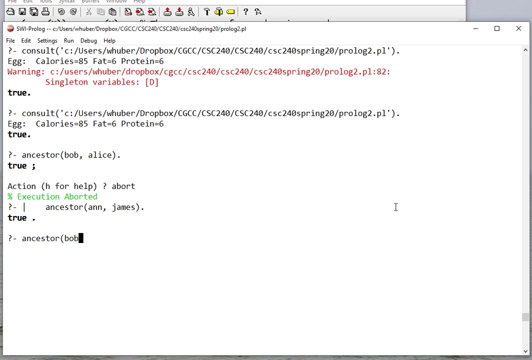 the mother of James, so that should hold the ancestor relation and that's true. so now let's check to see if Bob is the ancestor of suit. I don't think those will be ancestors because they both seem to have the same descendant, so and we have a infinite recursion. so the reason: 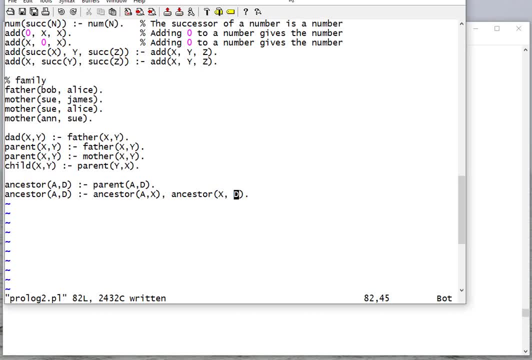 this is happening. I'll control C out of there. the reason that's happening is because this ancestor rule- we're just trying to find an ancestor ax and there's a lot of those, but then when we, when we do this relationship, we're saying ancestor, XD. well, finding either of these rules? notice, if there's not a parent relationship. 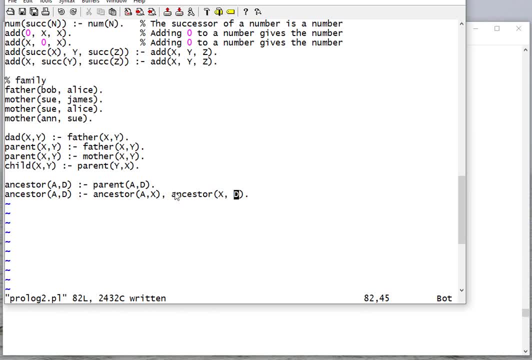 then this says: look for something else where that ancestor X is the ancestor of D. so I'm just going to keep trying all these combinations and eventually I'll get to a point where I'm flipping back and forth between two ancestor rules, and that's not going to be. 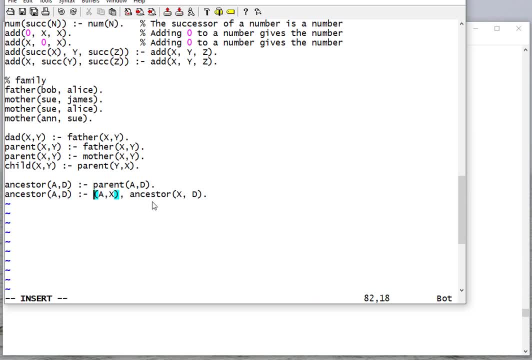 helpful. so to fix this I can say: parent ax and that grounds this first rule using the parent, this, this, this first clause using the parent rule, and so that way I'm only calling ancestor one time, so I don't get into a case where I'm going down some search path that I'm never gonna find something. 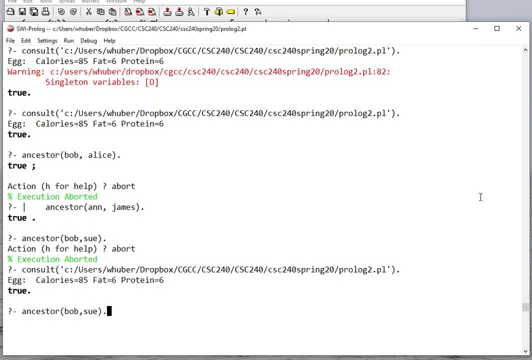 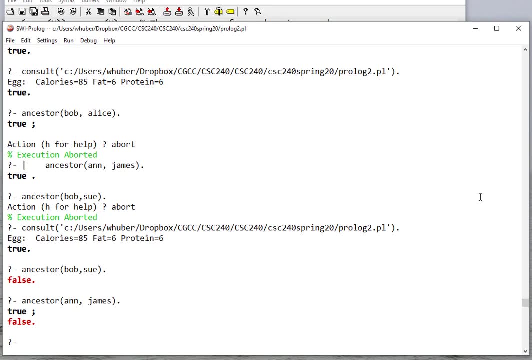 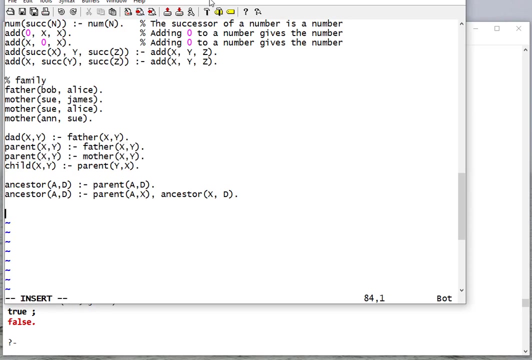 that works. so let's consult and let's see: ancestor Bob Sue is false and ancestor and James is true, and if I say no, it's gonna say false because okay, well, I found one path of ancestry but that's it. we can do something similar with graphs. 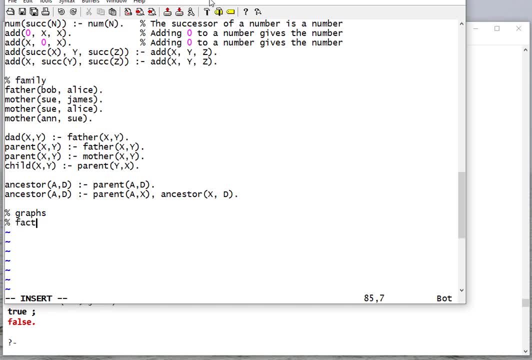 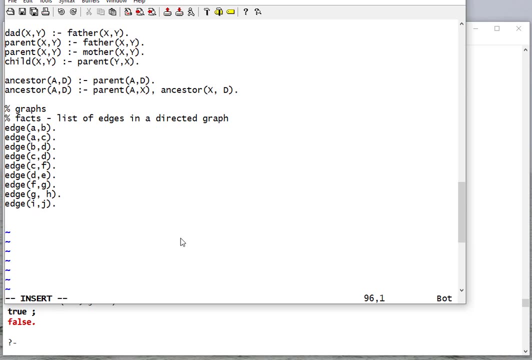 so we'll have some facts. that'll be a list of edges in a directed graph. sick, now I can do algorithms on on this graph. so, for example, I can say: a graph is connected. if there's an edge, what's colleges is those. You can have nano code, let's say 간다rus는. 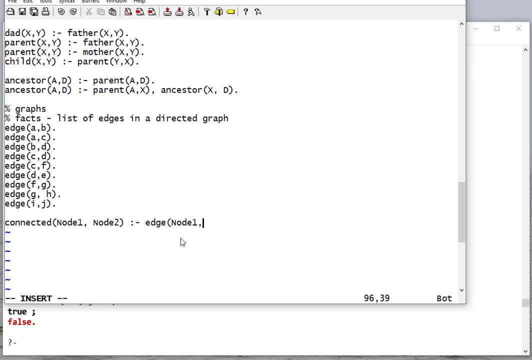 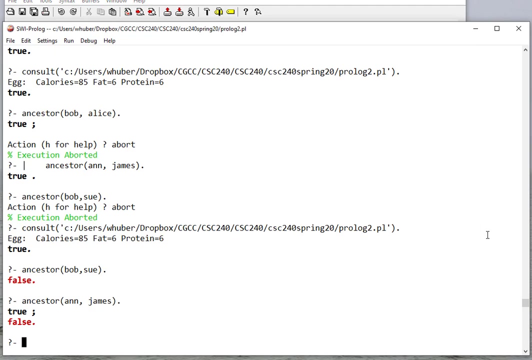 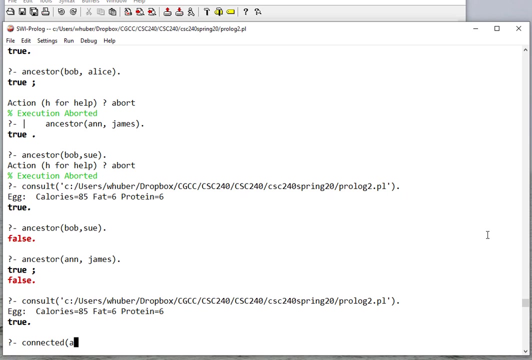 zięki number of AB股 pineapple from node 1 to node 2, or if there's an edge from some node x or node 1 to node x and node x is connected to node 2.. So if I consult, let's see what A is connected to. 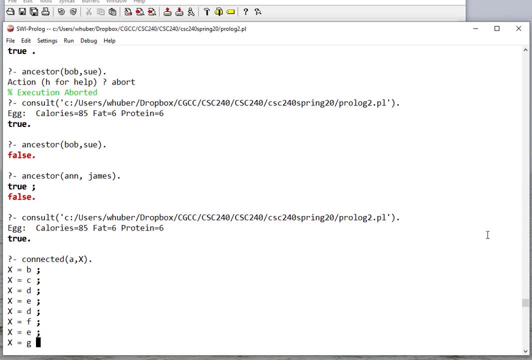 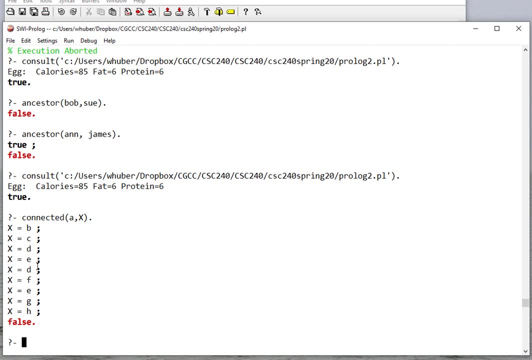 It's connected to B, C, D, E, D, F, and you'll notice I'm getting some repeats because that's again, it's basically finding a path from A to B, then C to D. Here we have a repeat because it found a different path to D than we found originally.